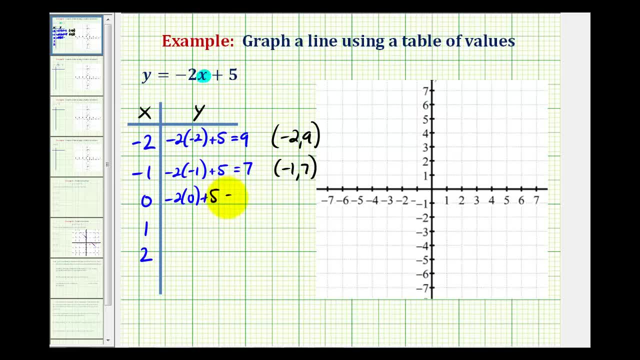 we'd have negative two times zero plus five, That's going to be five. So the line should contain the point zero five. And when x is positive one, we'd have negative two times one plus five. Well, this would be negative two plus five, That's positive three. 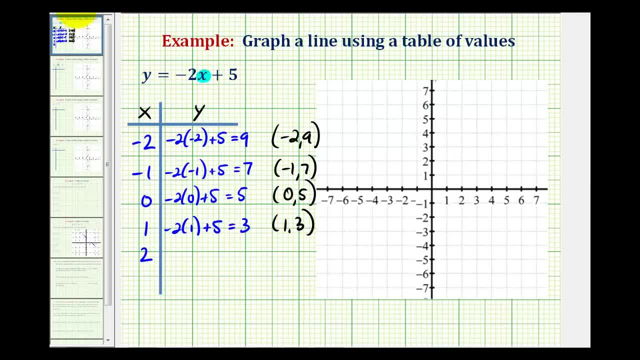 So the point one three should be on the line. And then the last x value we selected was positive two. So y is equal to negative two times two plus five. Well, this would be negative four plus five, which equals one. So the line should also contain the point two, one. 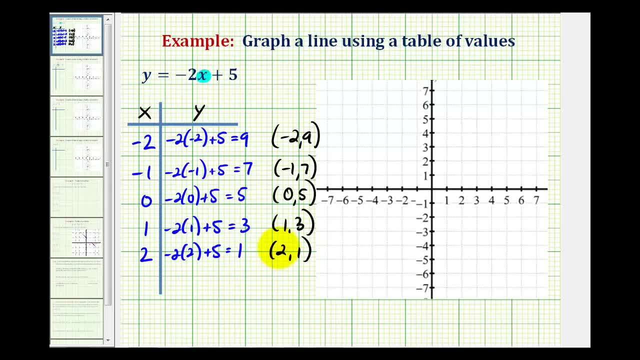 So now we'll go ahead and plot these five points and then sketch our line. So for the point negative two, nine, we'd move left two units and up nine units, which will be off the screen. It's going to be somewhere up here. 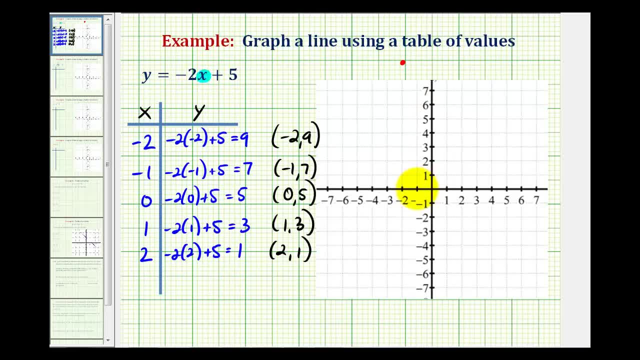 And then for the point negative, one, seven, we'll move left one unit and up seven units. Point zero five would be on the y-axis here. It's also the y-intercept of our line. For the point one, three, we'll move right one and up three. 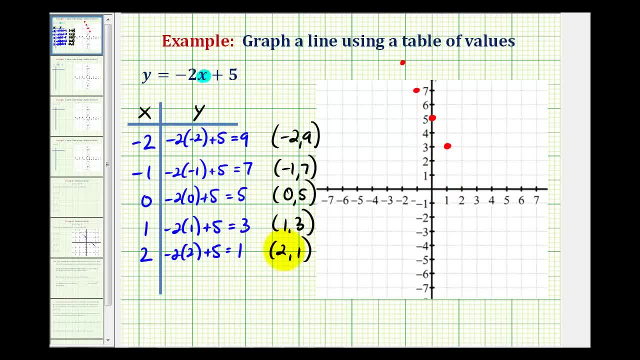 So right, one unit. up three units here. And the last point is two one. So we'll go right, two units and up one unit. Everything looks good here, because notice that all of these points line up to form a single line. So the graph of y equals negative two x plus five. 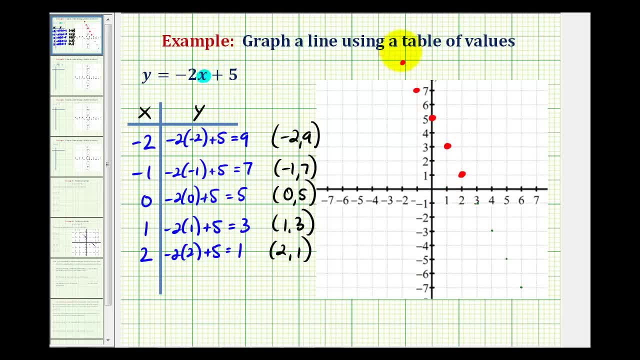 which would be the line passing through these five points. So it would look something like this. Now, I do want to emphasize that we could have selected any x value here and determined the corresponding y value, but these tend to be common x values to select. 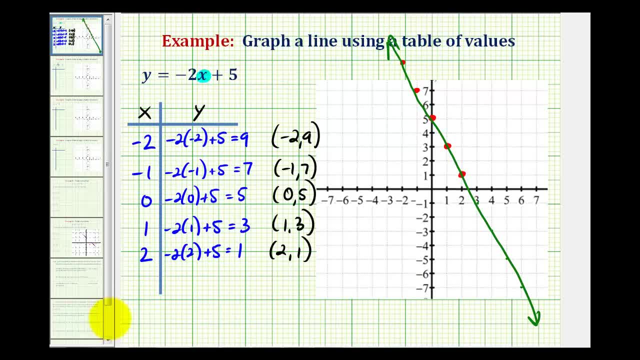 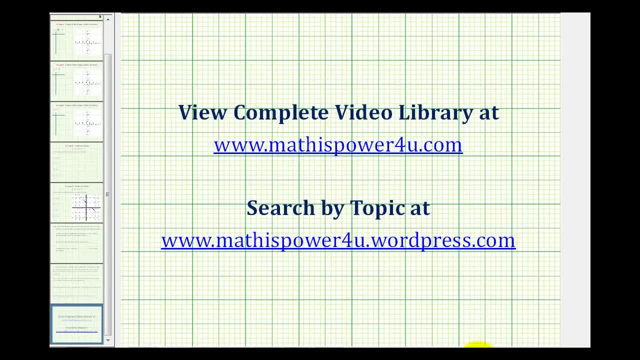 when graphing a line using a table of values. If I keep doing this in the middle of the graph, it will look a little bit more like this. So this is a negative 1, and if we lose this one, it will be a negative 1,.